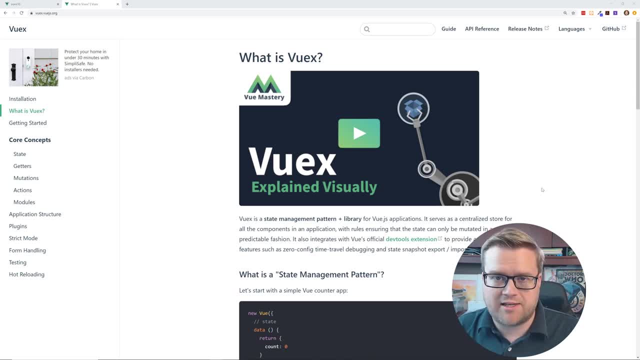 what Vuex is so if you're brand new Vuex is a state management library system for Vue.js it's based loosely on the flux patterns that you see in other libraries and frameworks so in react they have something called redux in angular they have something called ngRx so basically it's a way to 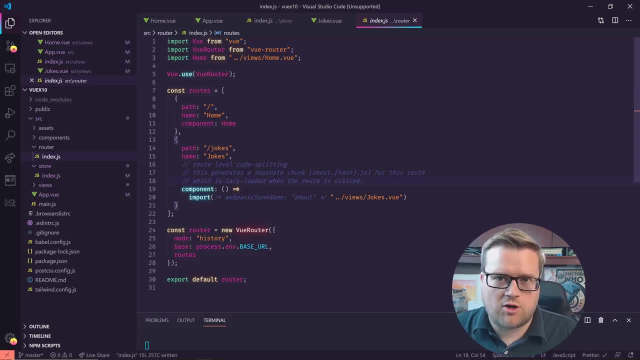 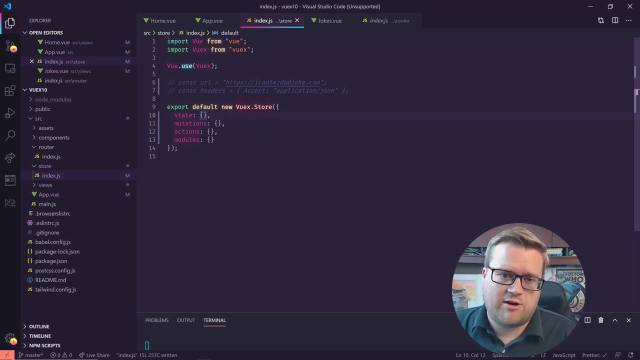 create a Vue.js application for your app so let's take a look so I went ahead and created a kind of an empty app for us to start so we can create our jokes app for us it's using Tailwind CSS it's also using just a vanilla Vue.cli app out of the box with a couple of changes I have a home route I have a jokes route and then I also have an empty store so I chose the option when I used Vue.cli to create it to create this store so let's see if we can go ahead and set up our store first so right 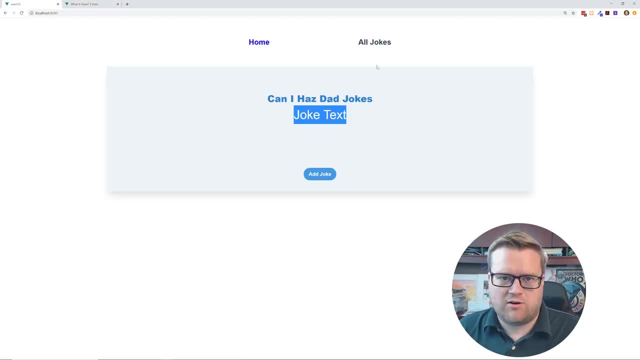 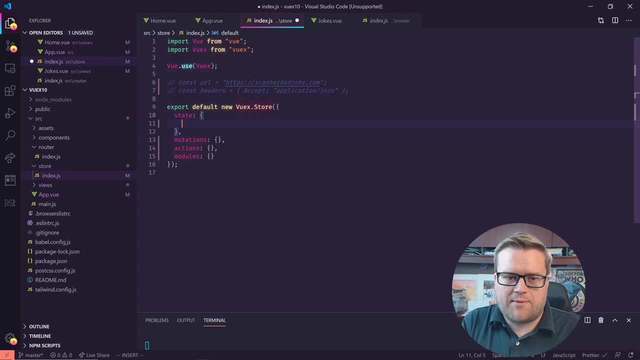 our app looks like this we have nothing in it this is just hard coded in and I just have some um just two routes right here like I was saying so what we want in our state and now state is the information that we're sharing throughout the app so we're going to create a couple of pieces of state first we're going to create joke current joke and this is just going to be an empty string and then we're going to do all jokes and this is going to be an array so we want to have every 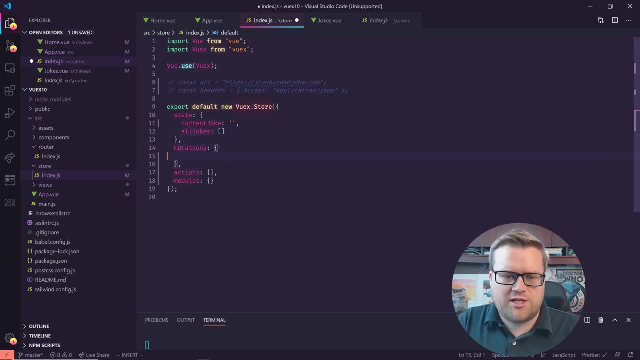 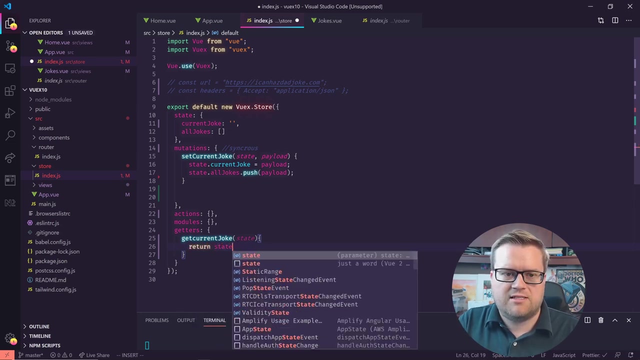 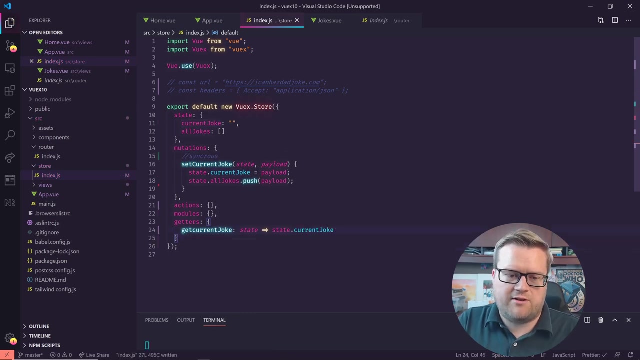 and then all our jokes displayed on our jokes route and then for mutations we want to actually set and change it so a mutation is a synchronous so I'll just make sure I put this here synchronous way to update the state in our Vue.x store so we can have set current joke and that has a state and payload that comes with it and then inside the same payload we can just set whatever we want so I'm going to use state dot current joke equals payload so that way the payload that we receive gets set into the state uh form for the Vue.x store and then we also want to add to the all jokes so I'm going to do state dot all jokes dot push because we know it's an array of the payload cool and now we want to look at one more that doesn't normally come in here is called uh getters and getters are a way that we can grab information and display it anywhere in our app and there's kind of nice things because we can kind of change things as we retrieve it so let's do get joke let's do get current joke and this has one option that comes with it it's called state and it just will return state dot current joke cool and also if we want to be fancy here we can actually do this kind of a arrow function here and then I can delete the return and then it's just a little bit more cleaner there so get current joke and that's just going to get 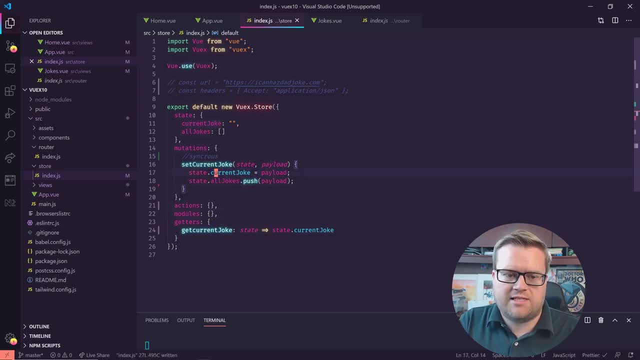 joke out of the state now right now all we're doing is we're setting this this up so let's say let's add a current joke in here this is a joke and let's see if we can retrieve this inside our app so we have this is a joke and i'm going to go ahead and just hide the sidebar 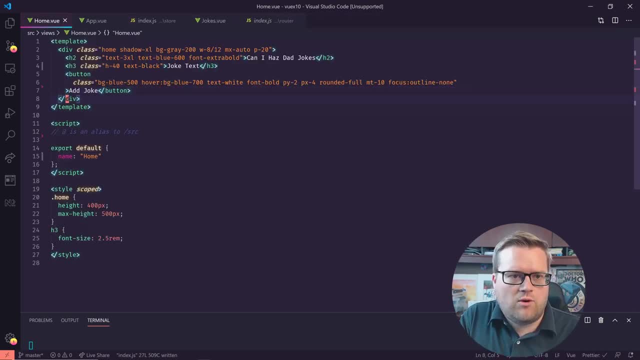 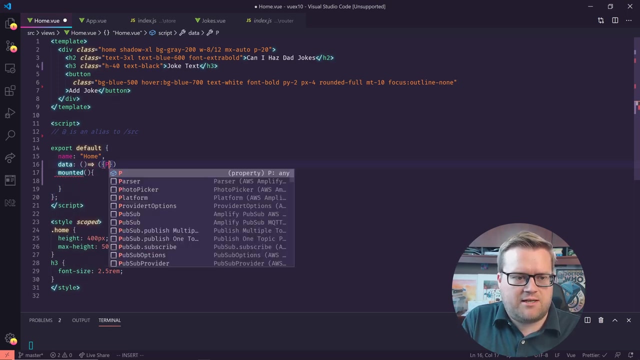 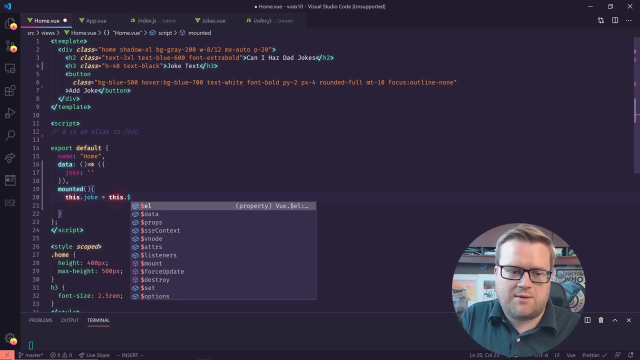 and now inside our home view we want to actually see this joke text we want to grab it instead of using this joke text here we want to grab it from the store so we can do that we can use something like a mounted hook and we're going to have a data object first and this data object is going to have a joke which is going to be an empty string but we're going to set this.joke to the store now one thing that's nice since we're using uh viewcli and and vuex is installed now we have an option to this dot store which has our access to the whole store at this point so we can do this dot store and then we can do getters dot get current 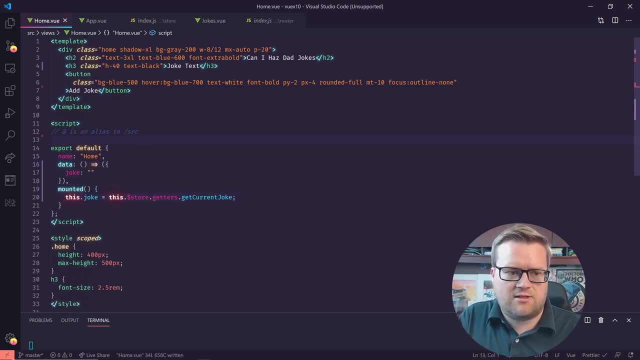 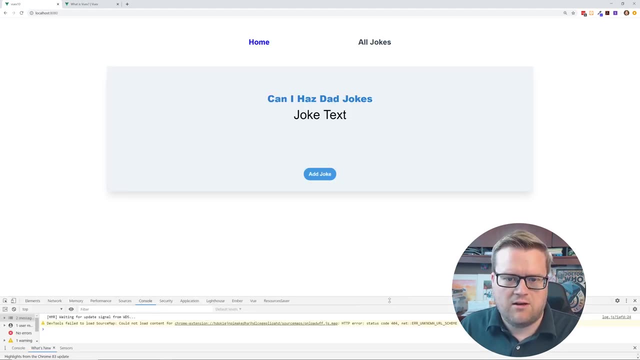 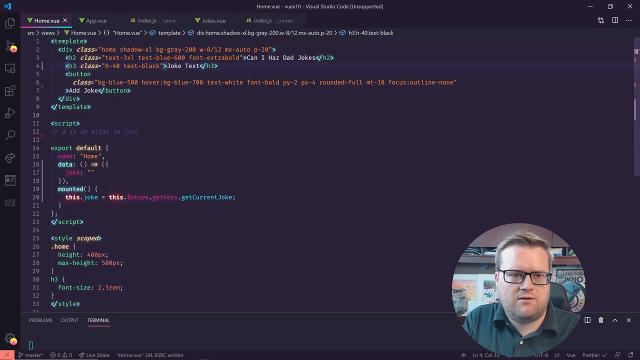 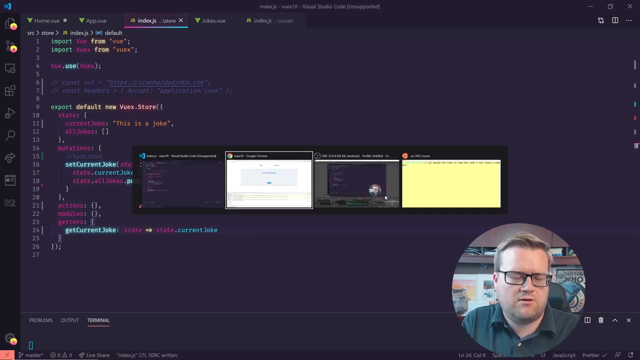 joke and that should update this dot joke so let's see if that worked so we see here because can i has dad jokes let's make sure we don't have any errors we can look at our console here cool so we have joke text in there uh let's make sure we update it so we're gonna put this to joke oh so one thing we mistake here we need to add in capital c current joke okay so it looks like it's retrieving it out of the store as we expected 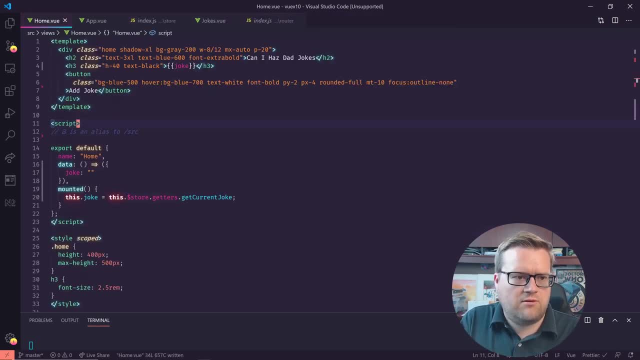 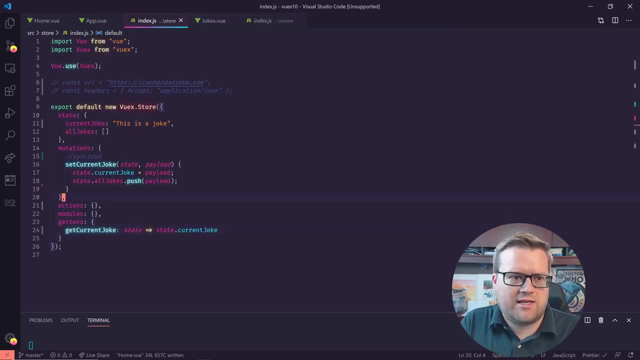 cool so if we go back to our home view now we have this is a joke so it's definitely grabbing the information out of the store but obviously we want to grab it from uh the actual uh api so i have an api in place so if you look at your index i already created this url and headers so there is a website called i can has jokes that i can grab information out of now you're probably thinking okay so maybe i can just add a mutation right here but since we're using api we're going to add a dichotomy and the way you want because of course like i said we don't need to and let's consider you know add empty cop Sebastian here so let's create a location and content so if I ahead of time use that and i'm at the end of the page what useful event is there something that i can use in order to to bring that conheced text in here like the journeys on it we can name it from here let's say emptiness yes that's a twit website and let's just save us that and i'm going to add like the physical answer in here and let's just see what happens with this let's speak to that like change this int guardians somehow in here to maintain that context so if we do that let's put a Heaventional Kathy so a patronx-based titan-theatrista So I'm going to call this const J joke, we'll call it joke, and then we'll do fetch. 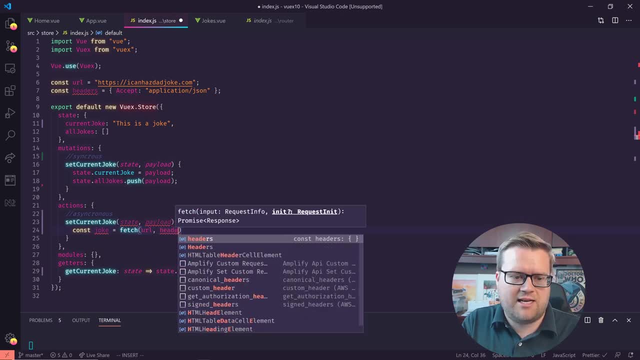 And since I already added in this URL up here, I can do URL and I have to do this headers here. 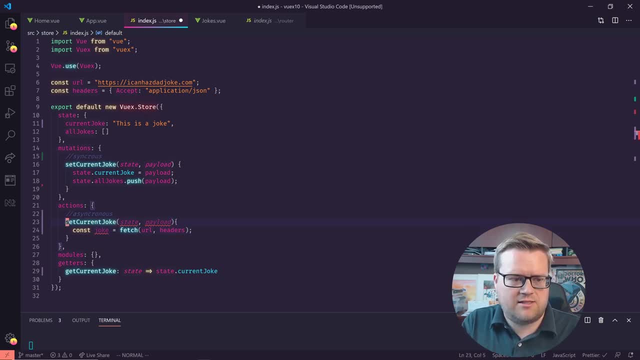 And just to make sure this works right, I'm going to make this asynchronous. So I'm going to do async here, and then I'm going to await the fetch. 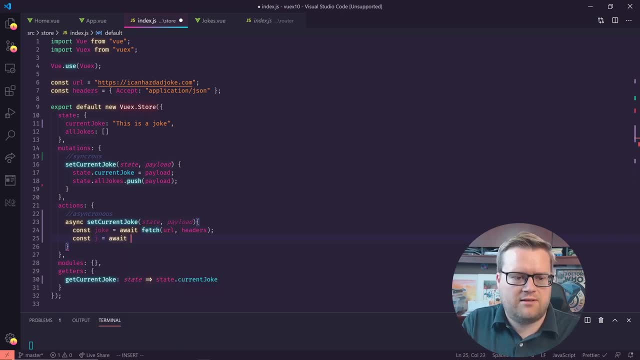 And then I'm going to const, and then I'm going to await joke.json. That should give me the JSON. 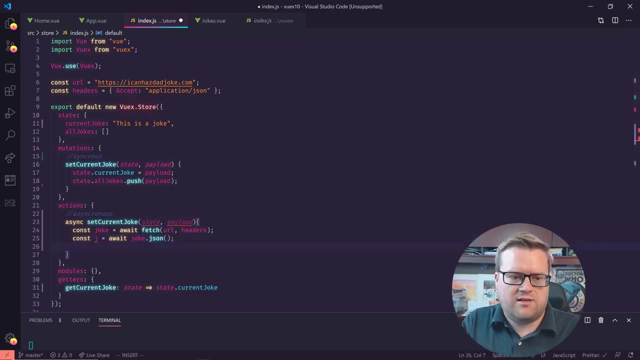 And now I can do something with this J, I can do state.commit. And so the reason I use commit is every time you want to change something in mutation, you do .commit. If you're trying to change an action, you do .dispatch. 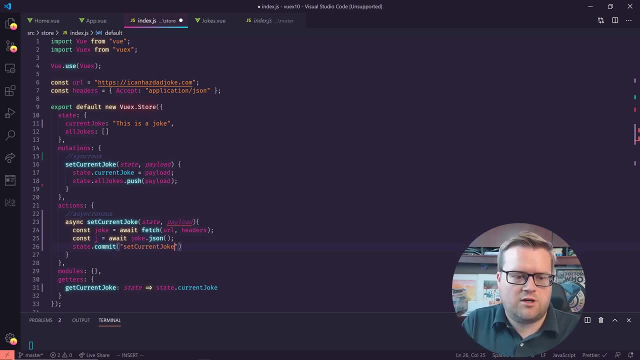 So I'll do state.commit, set current joke, and then I'll pass in J. And I know this has actually, it's an object called joke. 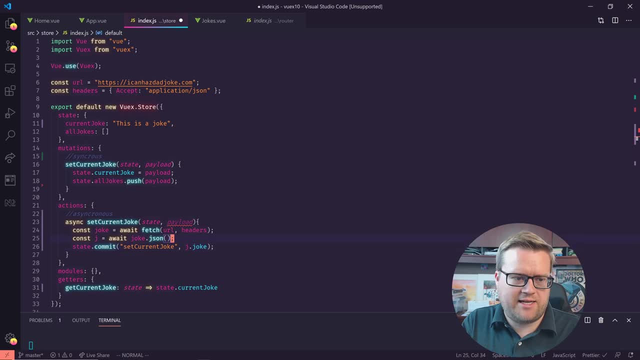 So we can do something like this. This should commit it into... To this mutation here. 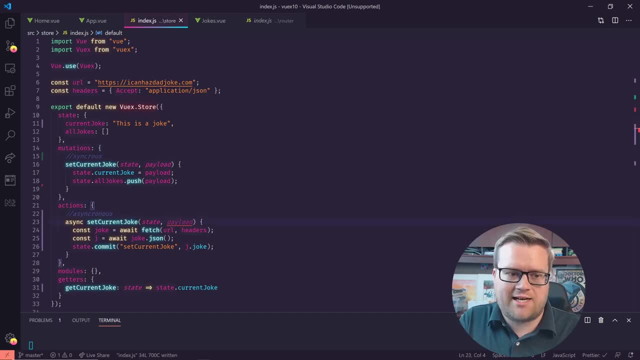 And now we want to see if we can actually trigger this action that we just created called set current joke. So to do that, I'm going to go into the app view. And I have this empty export default. 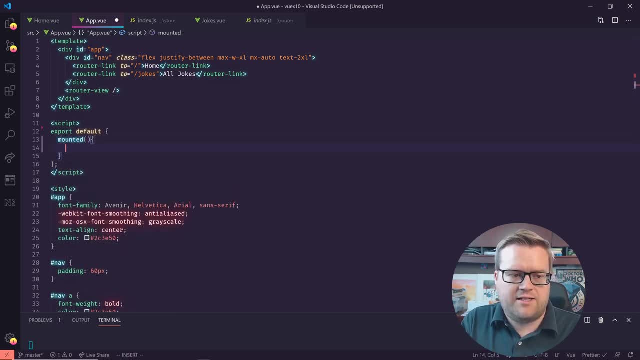 So I'm going to put a mounted hook here. And this time I'm going to actually trigger that action. So I'm going to do this $store. And I'm going to do commit. Excuse me, dispatch, because we're dispatching an action. And we know we called it set current joke. So we're going to go back to our app view, set current joke. And that's it. And one other thing we can do, we actually have this payload here. We're not using it. So I'm going to delete the payload. Oops, this is actually supposed to be an object. So try it again. Okay, so there's no errors. So now we've committed it. 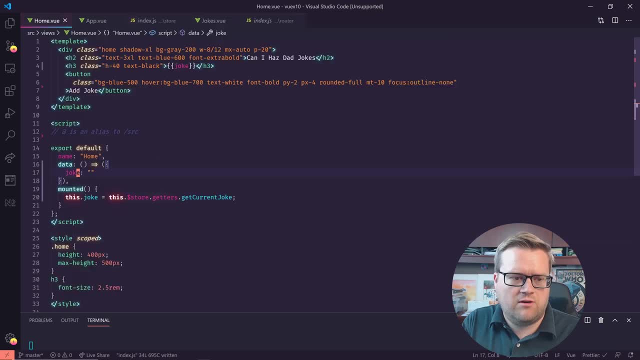 But now let's see, can we grab it inside our home view? So right now that you see, why isn't this working? We have them mounted. 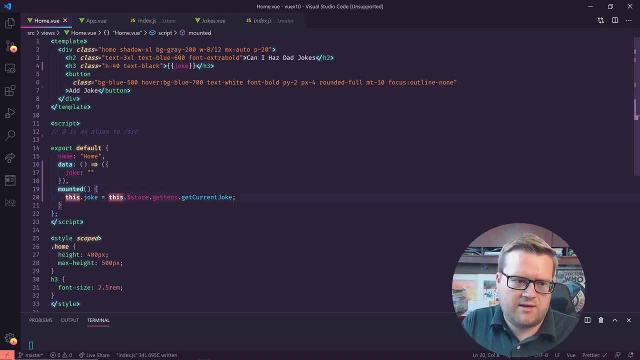 Because there's a timing issue. This mounted is being set before this app view is dispatching. 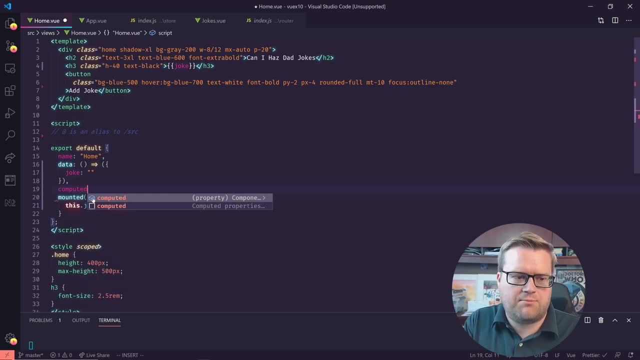 So if you ever run into this problem, what you want to do is use a computed property. So we're going to use a computed property. 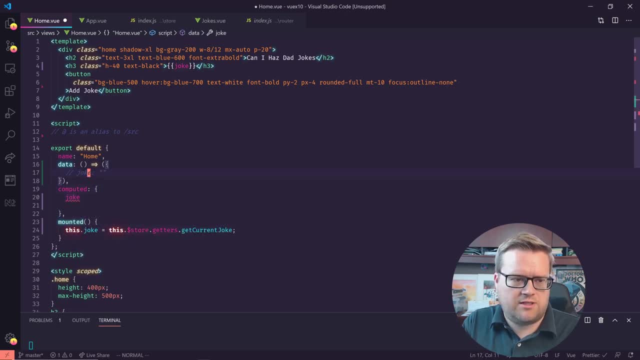 And we're going to call it joke. So I'm going to go ahead and just comment this joke out here. 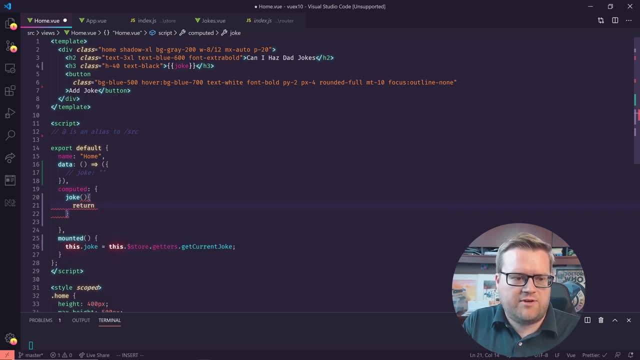 And this computed property is just going to return this.store.getters.get current joke. 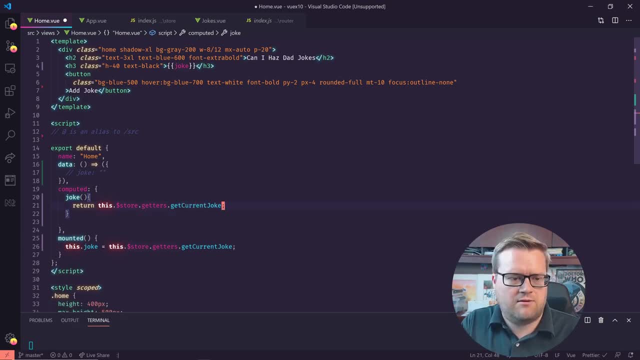 And then I'm going to go ahead and comment out this mounted right here. Cool. 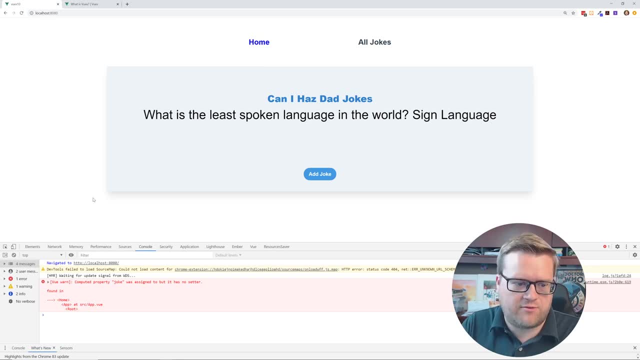 So now you can see here, it's actually loading the joke from the server. So if we refresh this, make sure everything's working, no errors. Cool. 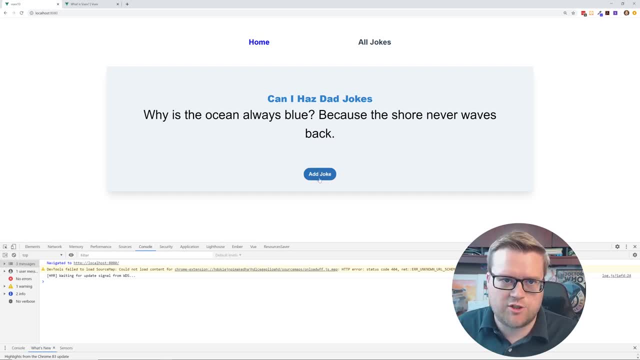 So we see you have it. Now we want to click this add joke and have a new joke appear every time you click it. So how do we do that? 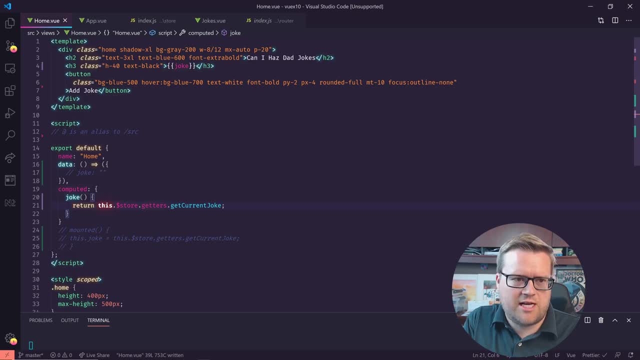 So we're going to go back here. Now, all this, all we're doing is, is just changing this computer here, but we want to add, do an ad joke. So I'm going to create a new, I'm going to go and delete the data right here. 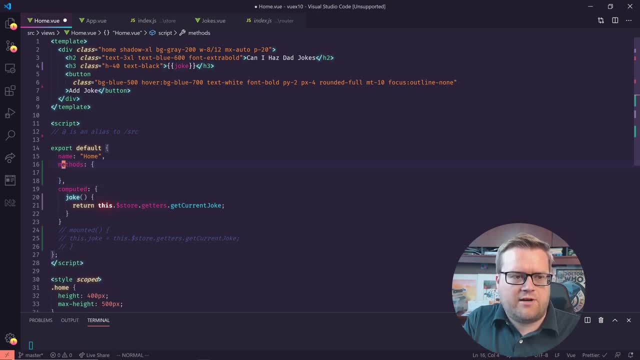 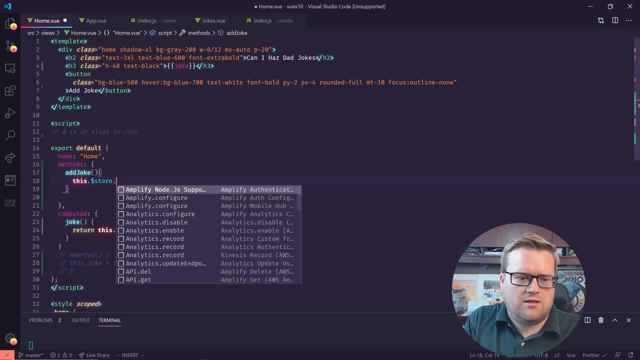 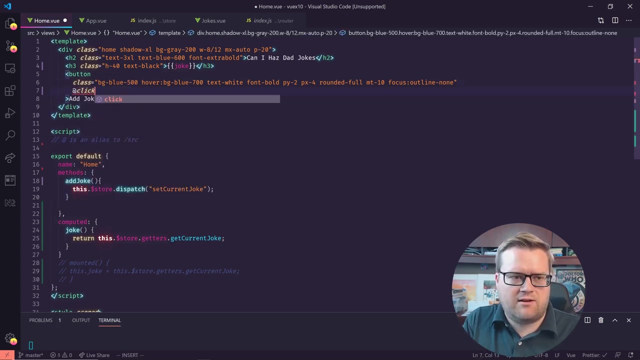 I'm going to create new methods and I'm going to create something called add joke. And note, this is going to do, it's going to just dispatch this, uh, this.store.dispatch. And we're just going to dispatch that set current joke. And so every time you click this button, so we're going to add a click event here. And just do joke. So every time you click it, it should do this. We'll call it, add joke, add joke. So every time you click it, it'll trigger this method here, which should dispatch that current joke, which should update the store for us. So let's see if it works. Click add joke. Cool. 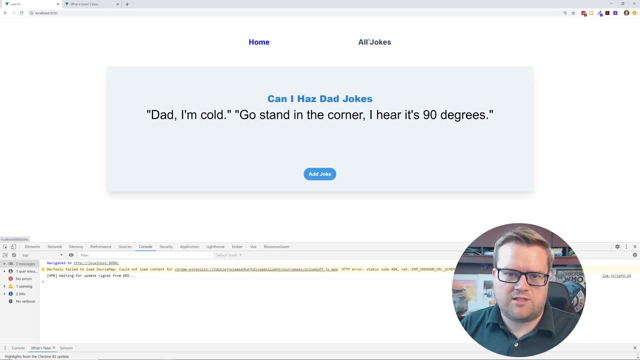 You can see here it's updating, but what about all jokes? So we still have our, all jokes. We just have this one joke hard coded in here. So how do we get all jokes working? So this should be easy. So we'll go. To our jokes route and we all, all we have is an export default here. 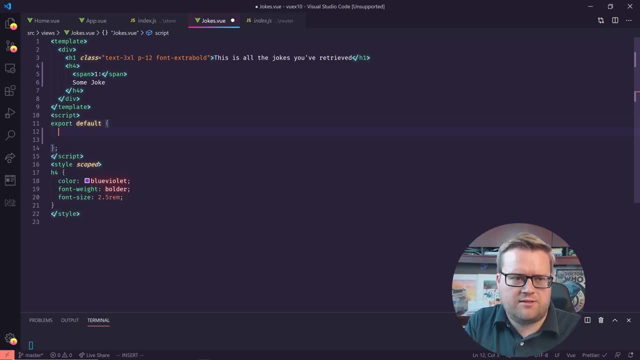 Um, but we can now retrieve all our jokes. So if we go back to our index file, so we have a way to grab current jokes. 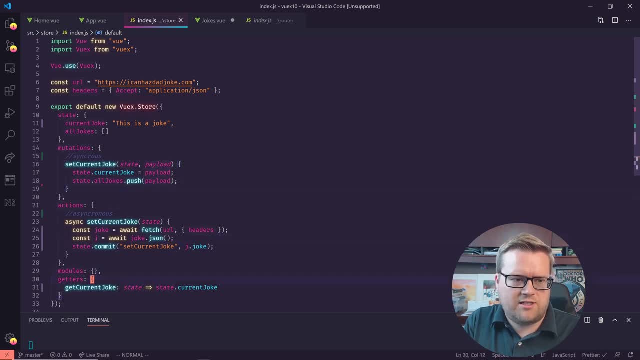 We're pushing to our all jokes. We're doing our actions and getters, everything's set up in here. 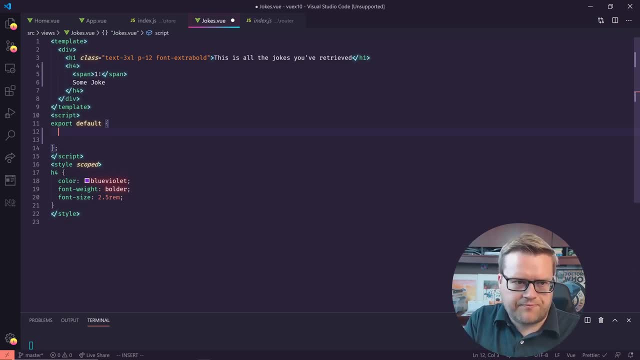 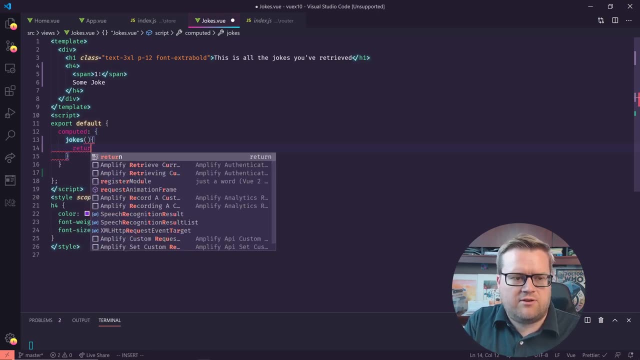 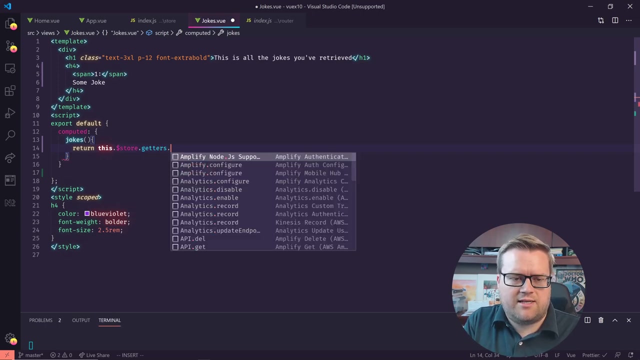 So I'm going to add in here, a, um, a computed property, and that's going to call, uh, I don't know. Jokes and that's, we're going to return, uh, this, this dot dollar sign store dot getters dot, uh, get all jokes. 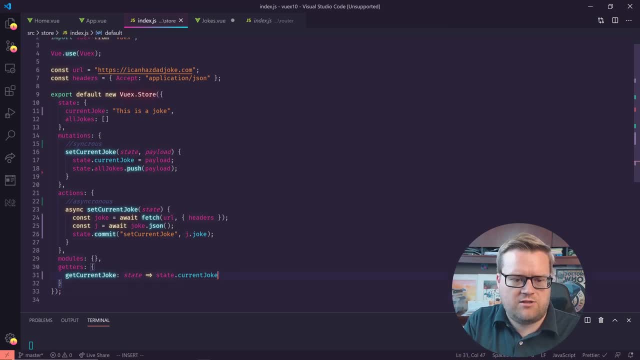 So if we look at the index file, we have current get current joke. So let's, let's set a new one. Get all, let's do get all jokes. 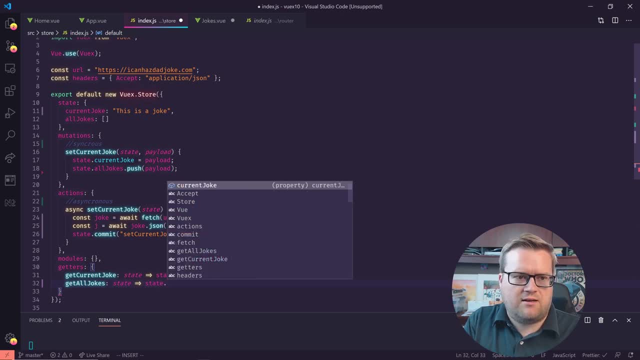 And that's just going to return state dot, uh, get all jokes. That should be it. Cool. 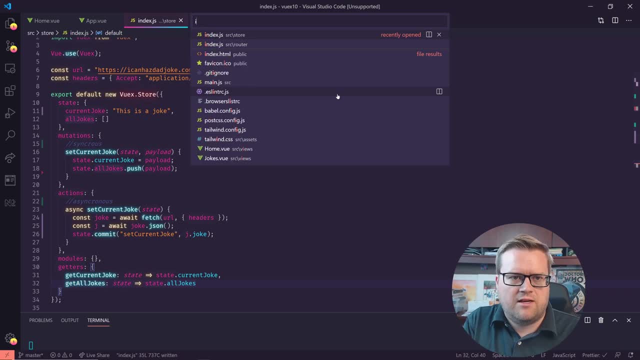 So now we have something called get all jokes. Now, if we go back to our jokes view, we can now should be able to do a V four in here. 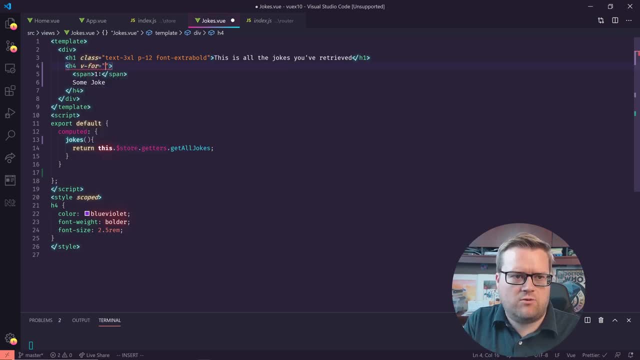 So we have this H four here. We're going to do V four equals joke in jokes. 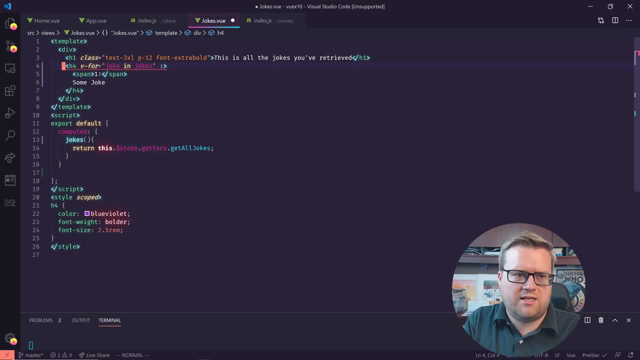 And remember, we have to do it. Um, we always have to put a key since we're using a V four here. So I'm going to do joke. End. Out. 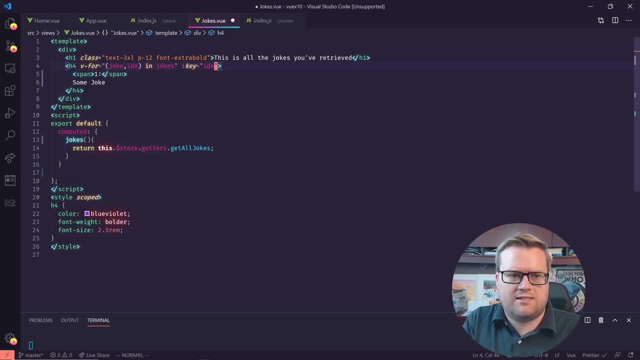 And then I'll do key here equals IDX. And now we should have access to this. So we can do here, this'll be IDX plus one. And then instead of here, we'll just do joke. 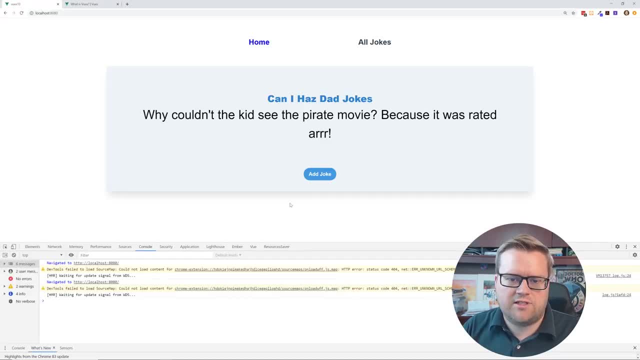 So let's see if that worked. So now we have our jokes here. 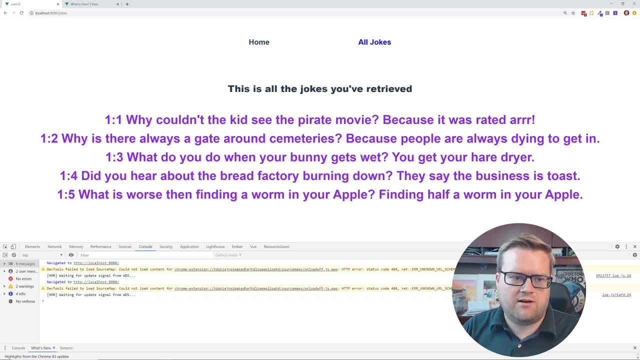 We can add jokes. And if you click all jokes, now they're appearing. Uh, it looks like we hard coded in the one there. I'll fix that. 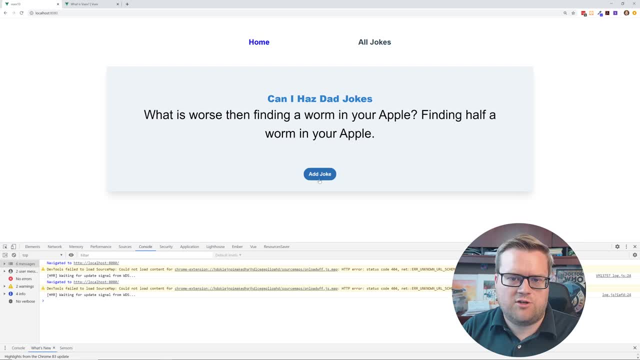 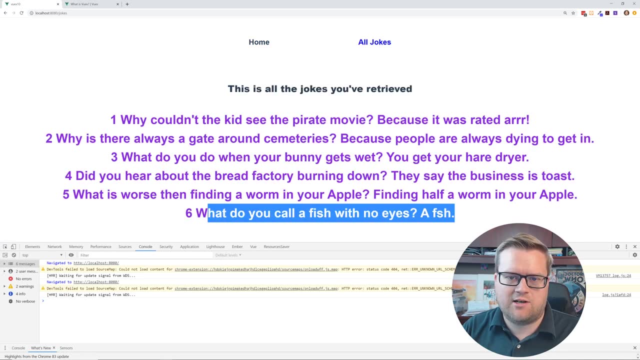 Yep. Here we go. So now we have all jokes. Now, every time you add a joke, what do you call a fish? No, I, uh, a fish says no, I in it, but, and now you can see here, and now it's listing in our all jokes page. Cool. 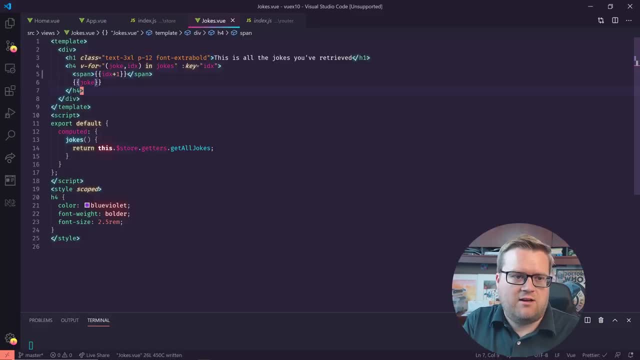 So we definitely did it, but we can make this a little cleaner. So we're kind of using this dot store everywhere, but there's actually view X helpers. 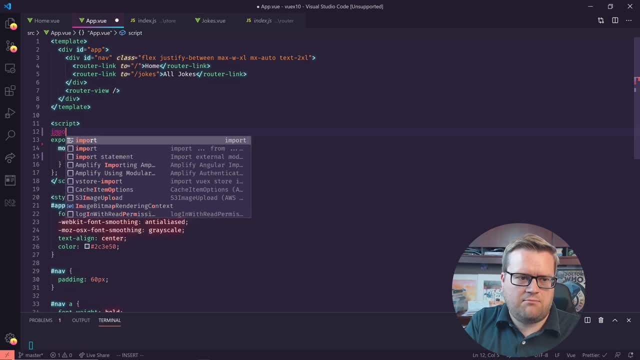 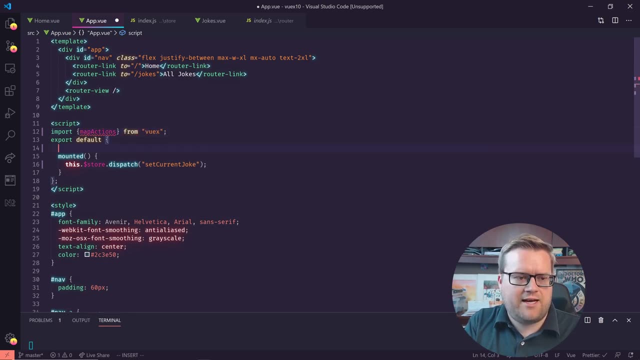 Um, instead of doing set current joke here, let's import map. Actions. From view X. And now we can do methods here and inside this map and methods, we can do app map actions, and then we can put in an array and this array would be set current joke. 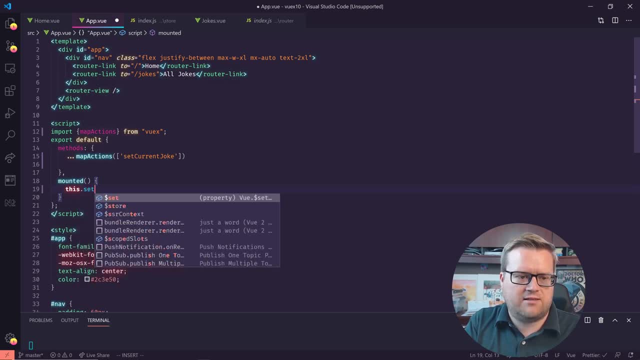 Instead of doing this dot store dispatch, we can do this dot set current joke and do it like this. So if we do like that. Yeah. 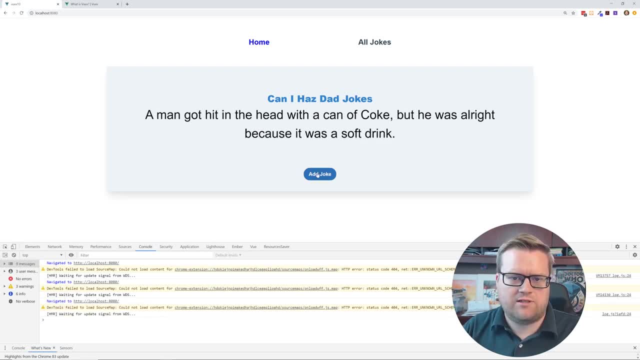 Let's see if it still works. Refreshing it. Cool. Still works. All right. 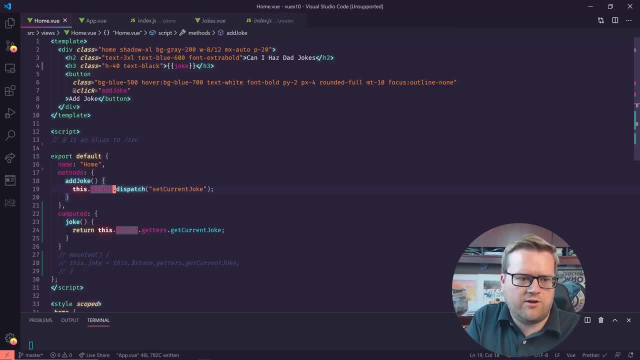 So we can do that everywhere. We can add these helpers everywhere so we can go to home view. 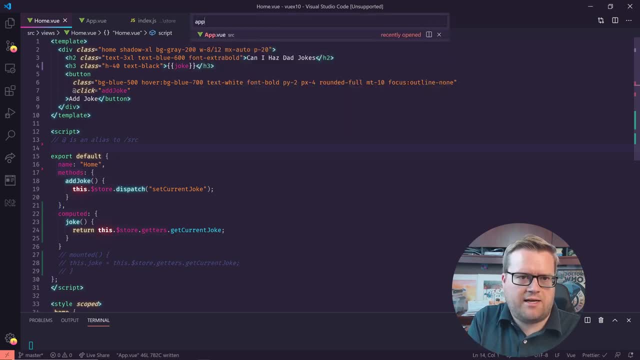 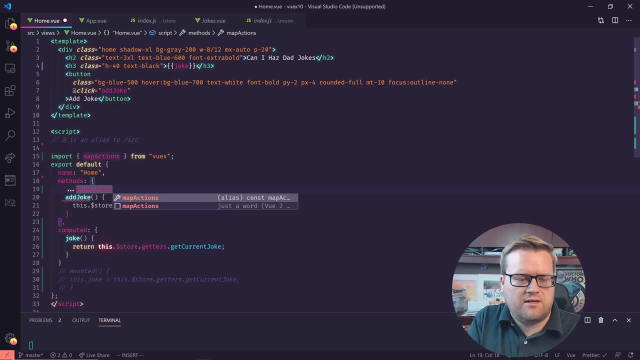 Um, we're once again, we're doing actions here, so I'm just go to my app view and copy and paste it and put it in my home view map actions. And then any side here, we'll have to put in the actions we want. So set current joke. And then instead of doing this. We'll do this dot set, current, current joke, and that, that should be it. So let's see if our ad joke still works. Cool. Still works. 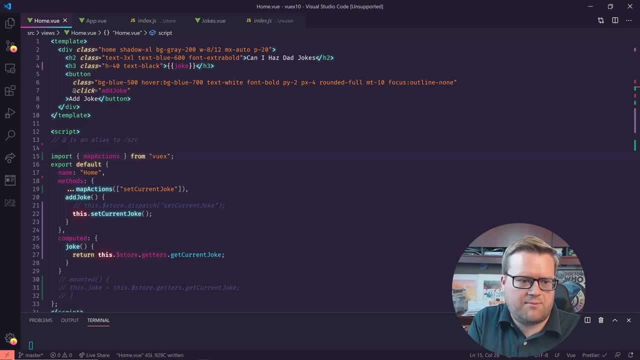 And we can do the same thing with this computer property. So instead of map actions, uh, we can do map getters, map getters. 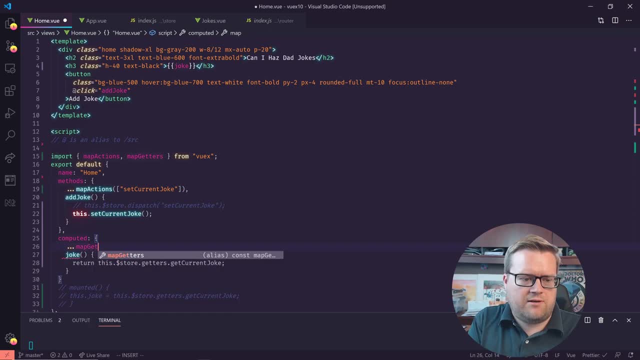 And in here we do the same thing. We, we do map getters here. 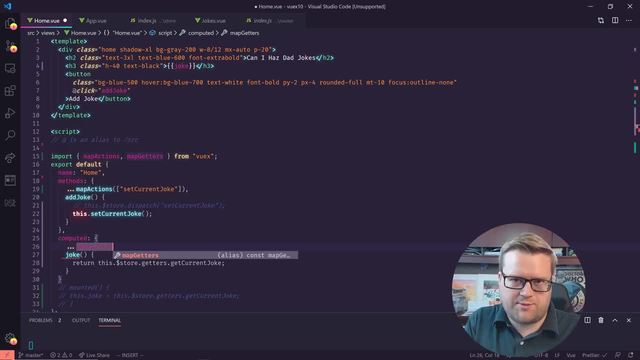 We do the three dots in front. In front of it, because we're using, we're spreading it, excuse me. 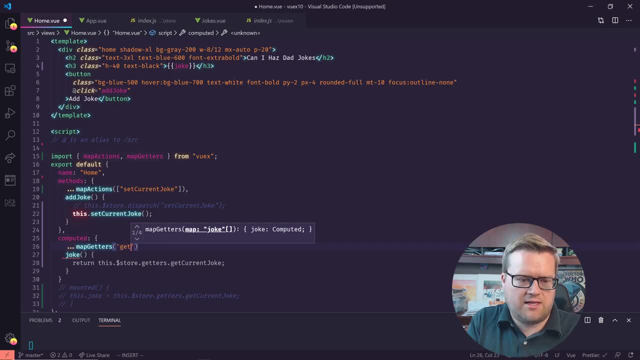 And then once again, now this is going to be a kind of a problem because we have something called get. 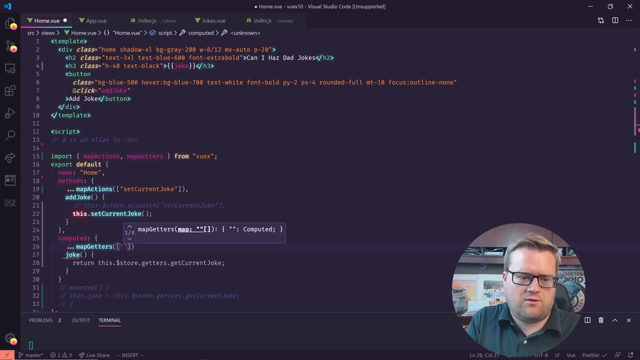 So if we put in an object here, it's always a method or it's either an object or an array, and we can do get current joke. 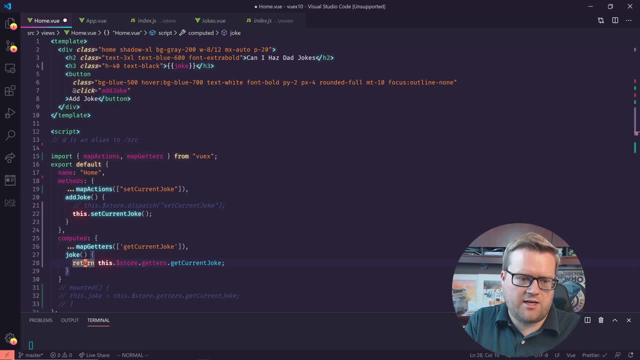 But the problem is now this, if we do this return here, we're returning this store dot getters dot current joke. So we could do this, um, instead of this store, store getters, we can do 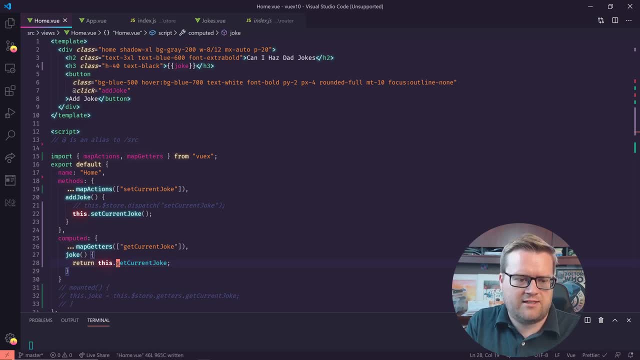 return this dot get current joke like this, and this would work. Uh, so if you go back here, so this is all working here in our home view. 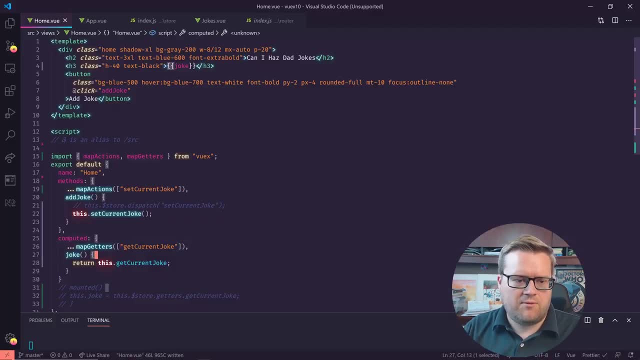 We, um, add it here, but it probably would make more sense that instead of this joke here being this dot current joke, we wouldn't want to have this method at all. 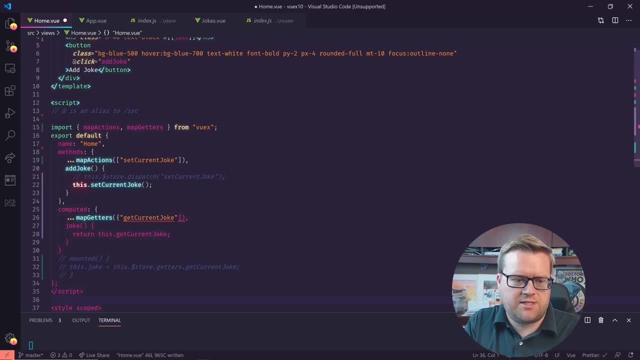 So there's something we can do here. We can change this to an object. Oops. So we changed. This to an object. 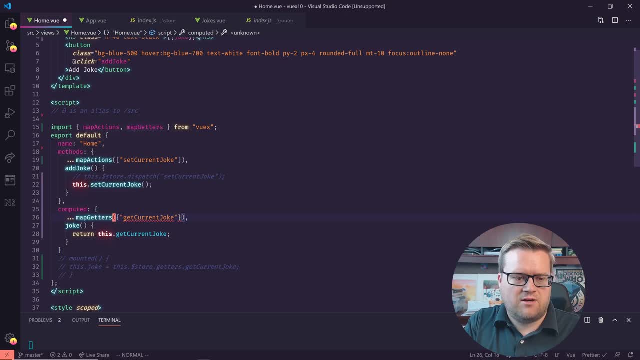 If I can do this, right. And then in this object, we just, you can set the name of it. So I just want to call this joke and then I can just comment this out. 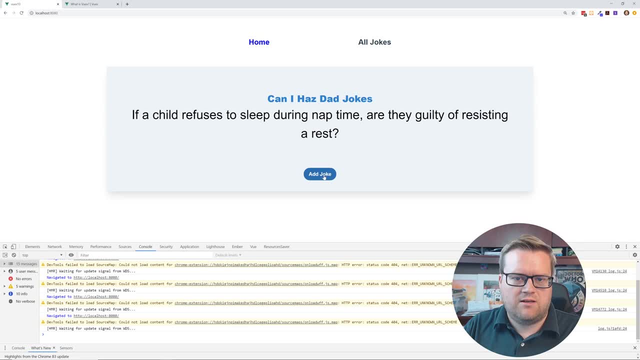 And now if we come up here, refresh it, see, it's still working. 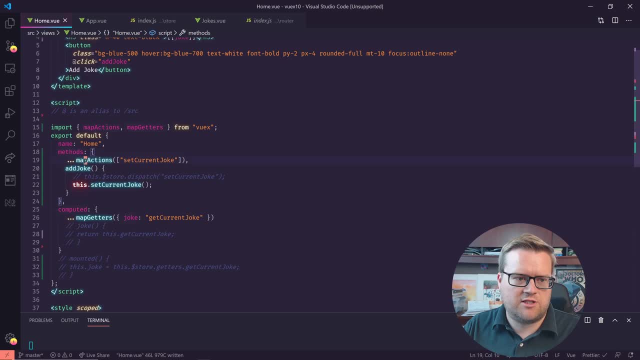 So cool. So now we've gotten, made it a little bit simpler, but what about this set current joke? Could we do the same thing here? So instead of. Um, we have this ad joke button here. 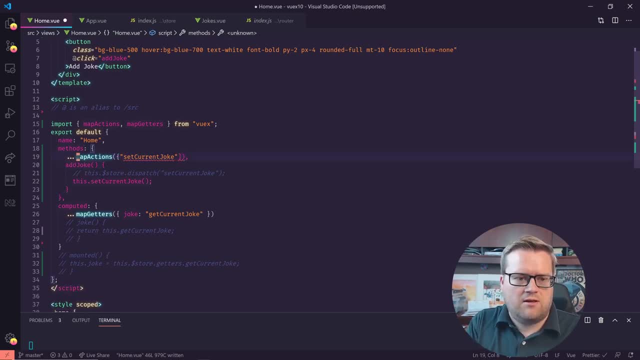 So what happens if we do this, we change this to an object. Let's see here. This is an object. 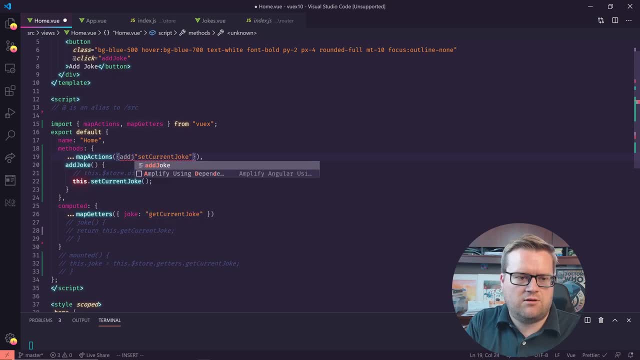 And then we call this ad joke, ad joke like this. 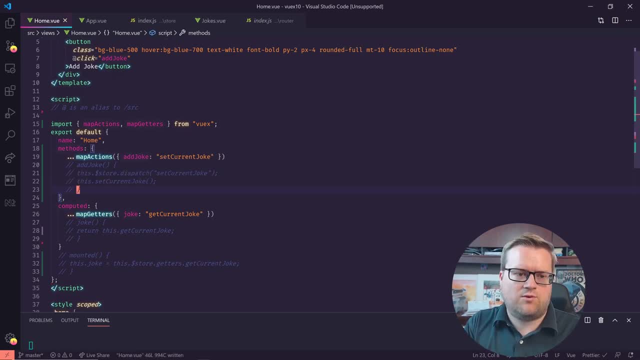 And we comment out this. Let's see if it still works. Yep. It's still working as you expected. So we haven't broken anything, which is really cool. 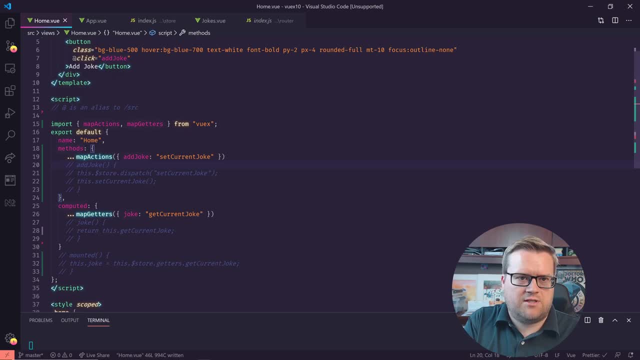 And now we don't have to have these extra methods here. Awesome. So the last one would be jokes view. And same thing here. It's usually, if it's just one, it's not that big of a deal. Okay. 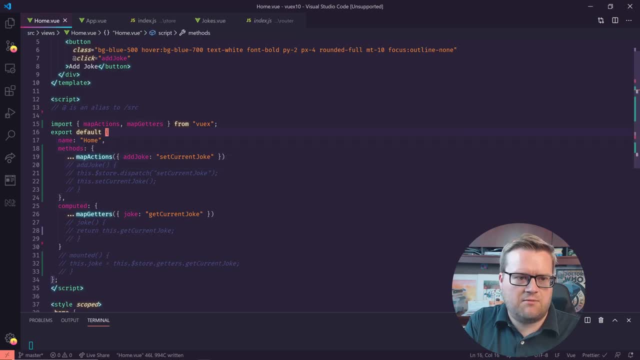 So we're doing, uh, same thing here with the getter. So I'm just going to copy and paste this into our jokes view. And we just need map getters. Cause that's all we have in here. 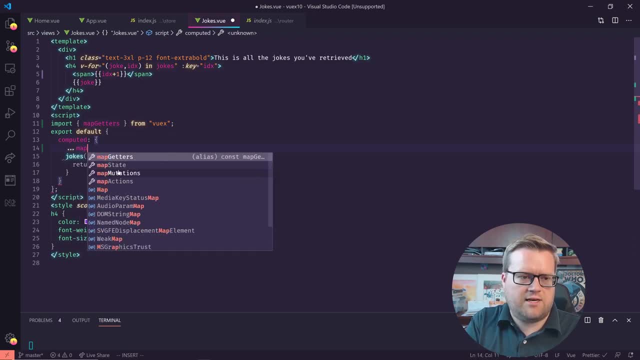 And then instead of this jokes here, we're going to do this map getters. And then we're going to have an object inside of it. And inside that object, we're going to call this jokes, and that's going to be part of get all. Jokes. And just to fix this, we'll fix it like this. Cool. So let's see if that worked. So refreshing it, add joke, all jokes, cool, still seems to be working. All right. So you, that is basically it. So we've used Vuex methods, we've used actions, we've used mutations, we use getters, we used all the things you should know for Vuex. If you guys liked this video, make sure you click that subscribe button below, and I'll see you in the next one. 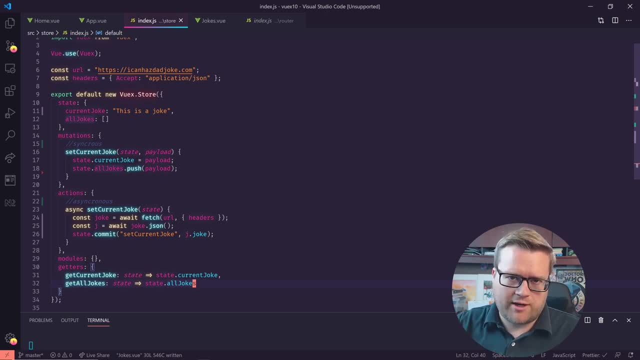 And also I have a course on Vue. I'll go ahead and put a link in the description below. If you click on it, I'll let you know next time it's available and you can sign up. So I really appreciate it. If you guys like these videos, here are some other videos may like, go ahead and click on them. I really appreciate it. Thanks. Thanks for watching! 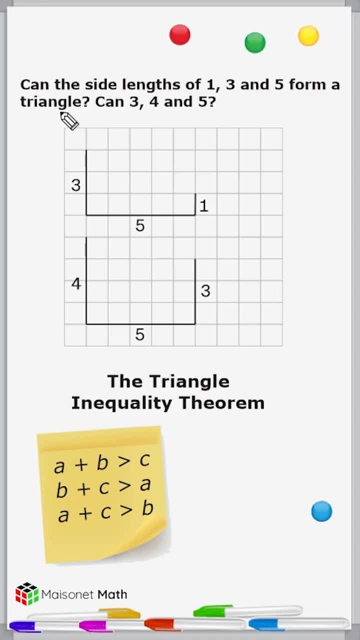 Alright, we have to determine if the side lengths of 1,, 3, and 5 can form a triangle, and we have to do the same thing with the side lengths of 3,, 4, and 5.. The triangle inequality theorem states that if you add any two sides of any triangle,